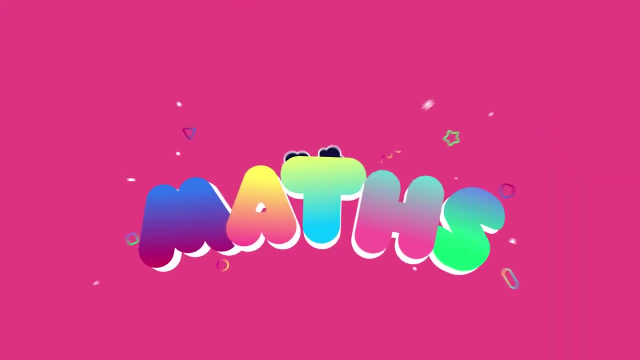 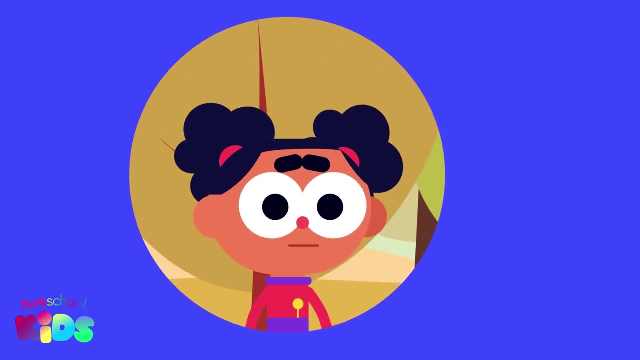 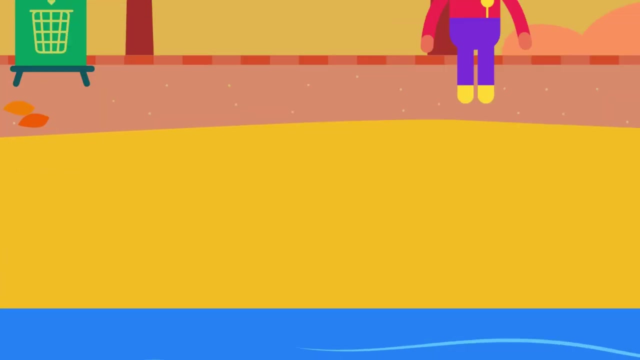 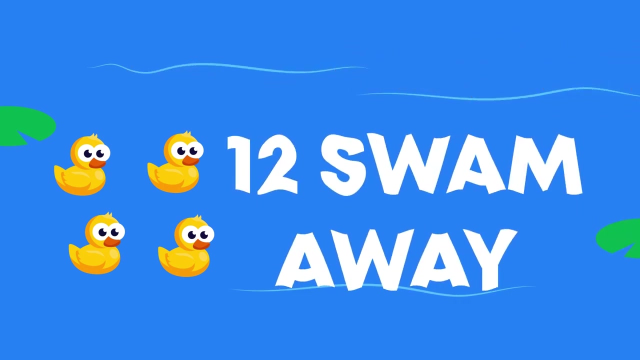 Hi everybody, I'm Ava. Today we're going to use different tools to help us subtract or minus with bigger numbers at the park. Let's try it. Aww, look at the 16 little ducklings. 12 of them just swam away. 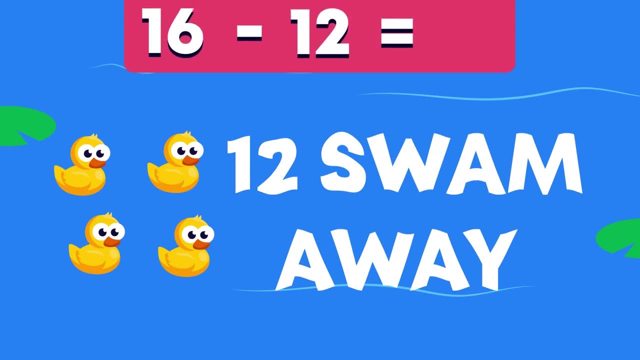 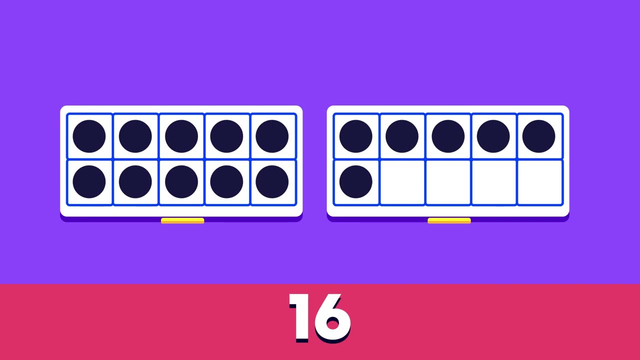 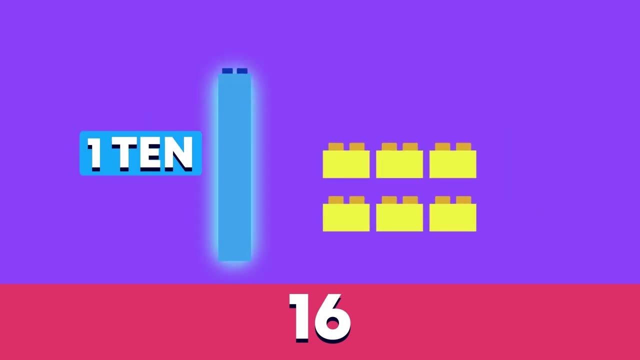 To find out how many are left, we can work out 16 minus 12.. There were 16 ducklings, so we start by showing 16.. We can use a tens frame like this: 16 has one ten and six ones. 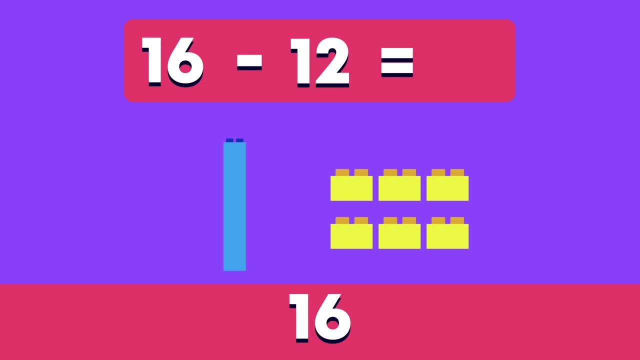 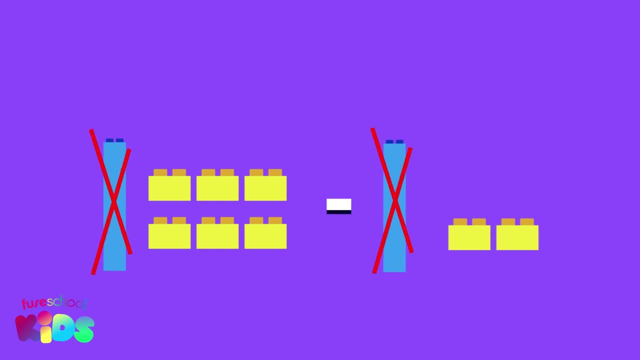 Now we need to take away 12 from 16.. 12 has one ten and two ones. We need to take away one ten like this and two ones like this. What is 16 minus 12?? It's 4.. Super, subtracting everyone. 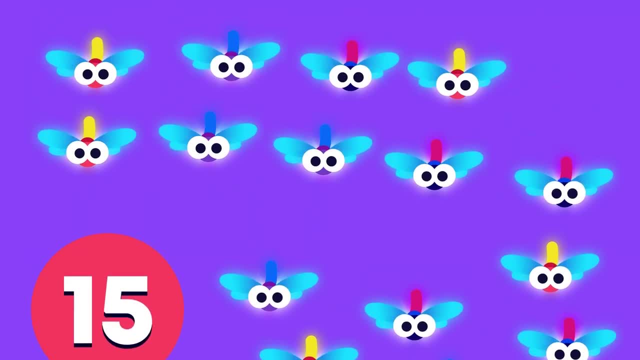 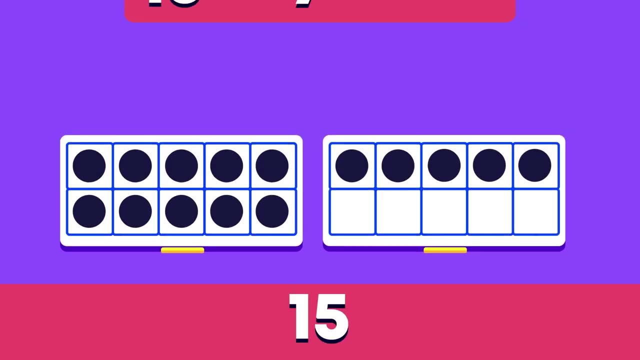 Look at the 15 shiny dragonflies. Oh no, 7 flew away. Let's use the tens frame again to help us work out 15 minus 7.. We started with 15. 15, so we build 15 like this. 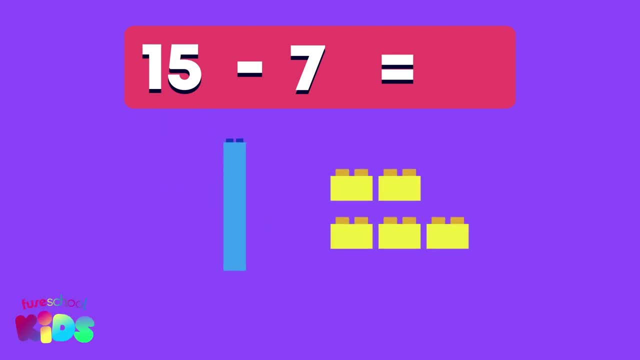 We need to take away 7.. We start by taking away from the tens frame. that is not complete like this: 1, 2,, 3, 4, 5.. Are we finished with our subtraction? No, that's right, Let's keep taking away. 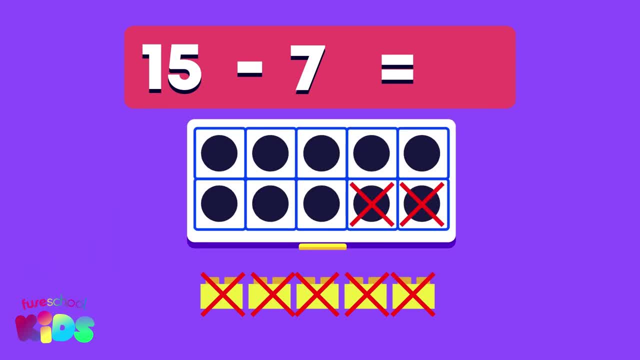 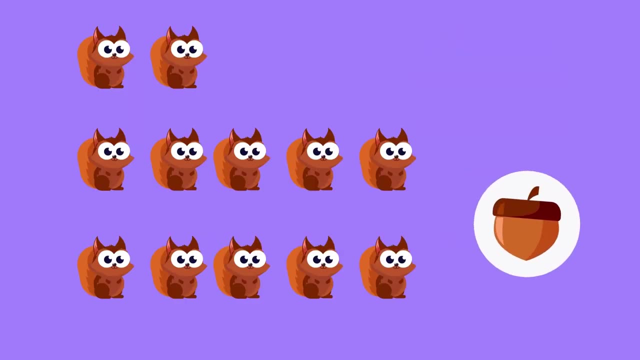 6, 7, so So what is 15 minus 7?? We have 8 left over. Well done, Ouch. There are 12 squirrels and 7 acorns. The squirrels want to know how many more acorns they need so that they can each have 1.. 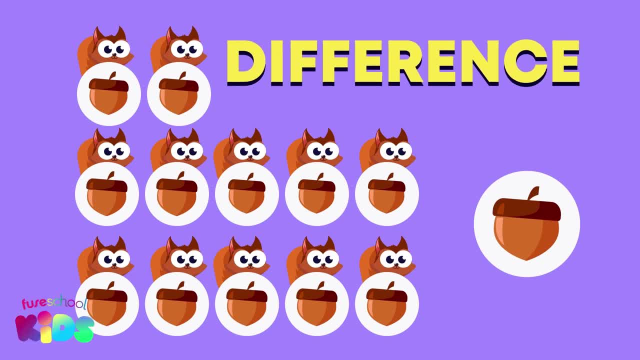 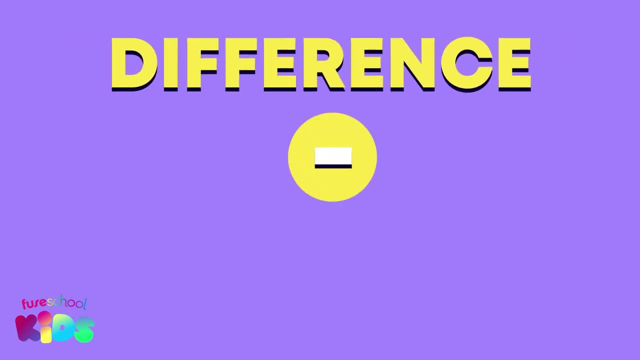 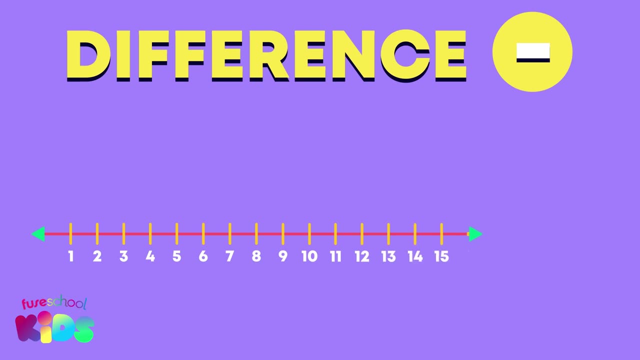 This is a different sum because we want to find out how many more we need to get from 7 to 12.. Remember, difference also means subtraction. To find the difference, or how many more, we can count up from the smaller number using the number line.